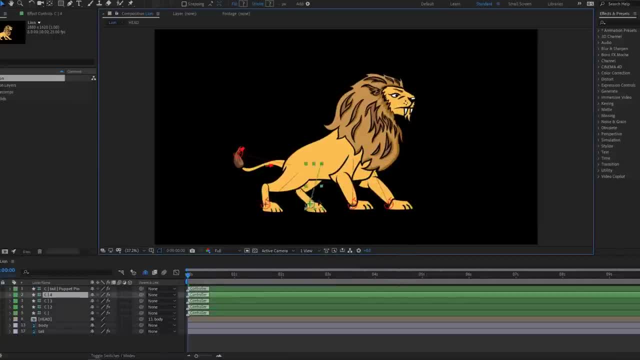 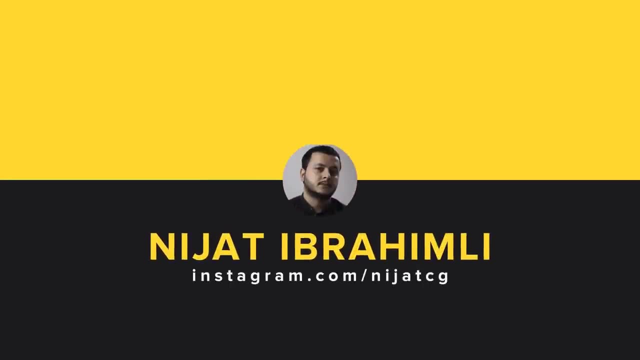 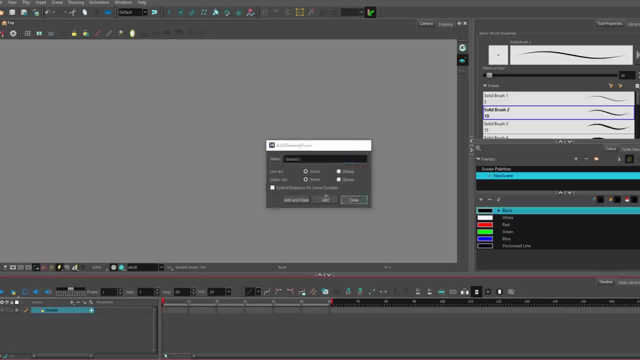 Before starting this video, you can like the video and subscribe to our channel to support us. Let's go, Number 1. Toon Boom Harmony. This software is specialized about 2D. Several 2D cartoons are made by Toon Boom so far. 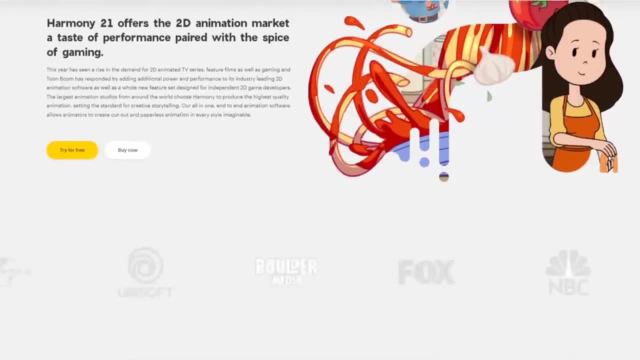 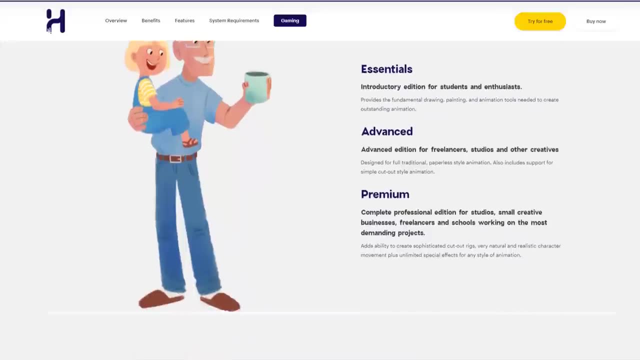 and currently they are being made by Toon Boom Harmony. It is possible to make square-square animations in the software. If you are drawing well, this feature is for you. Of course, rig system is available. You can get well results with making. 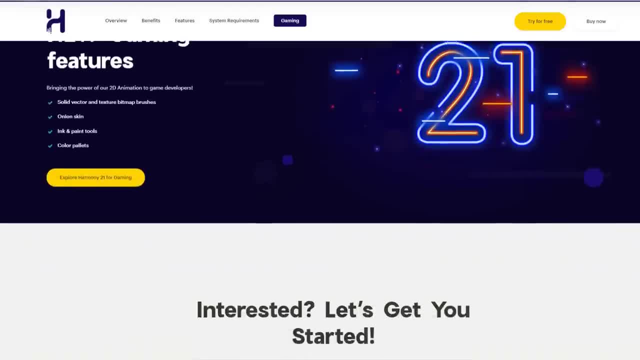 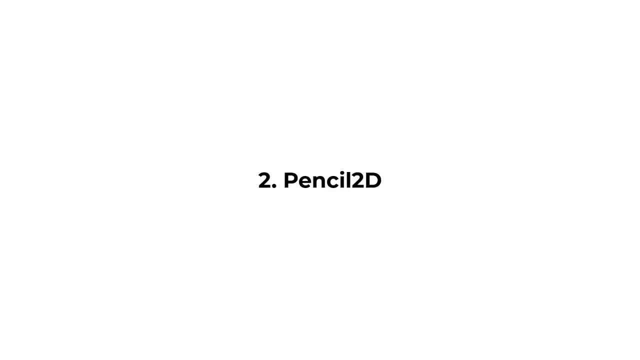 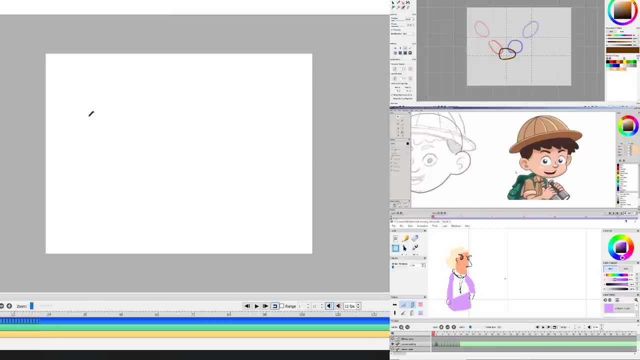 rigged drawn characters. So you need to use this software if you want to be a 2D expert Number 2. Pencil 2D: You can make vectorial drawings with beautiful animations in this software. Thanks to this software's basic interface, we can make our animations easily. 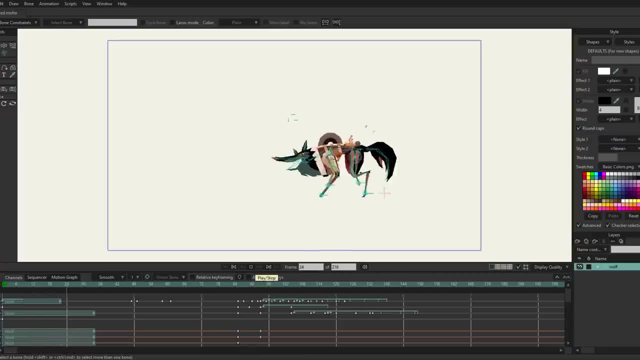 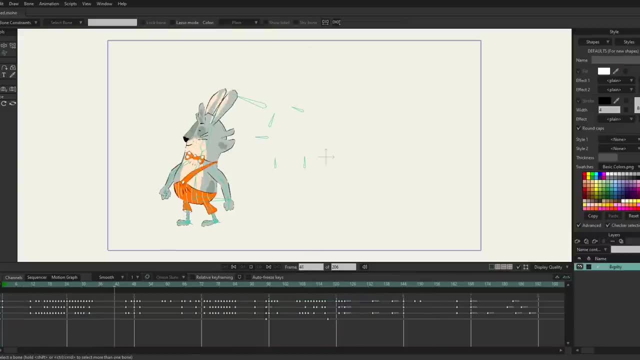 Number 3. Moho Pro. Moho is an animation king. Yeah, you heard it right. Features which inside the Moho make it the king. Many animation features and easiness drives it forward. You can make easy and fast animation with fantastic character rig making and dynamics. 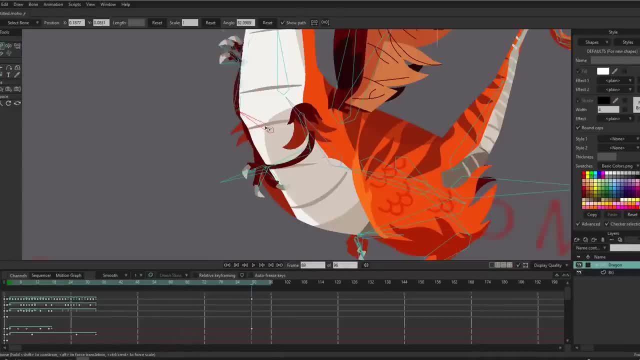 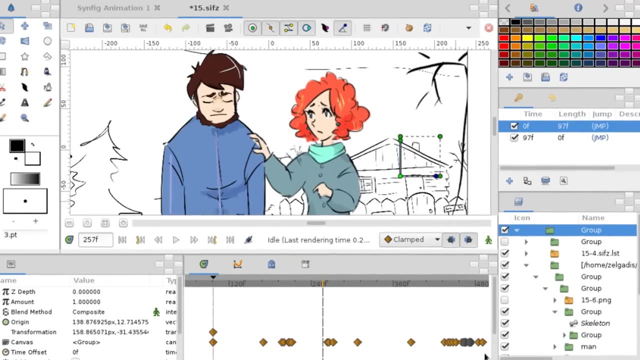 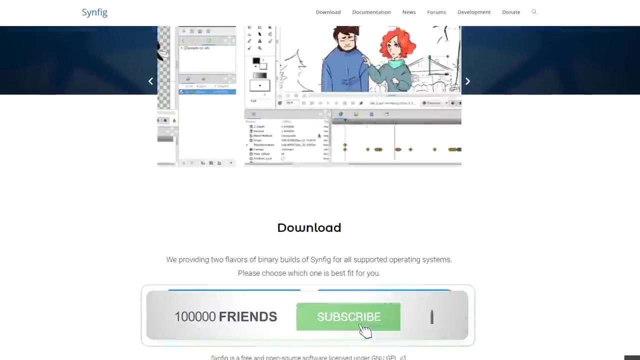 If your dream is to be a 2D artist, you must choose Moho Pro 4. Sinfig, As you know, for a classical 2D animation, you need to draw every frame one by one. For example, if a character is walking, you need to draw each frame of the character. 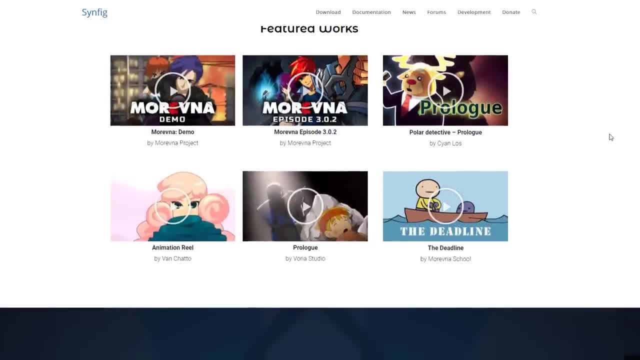 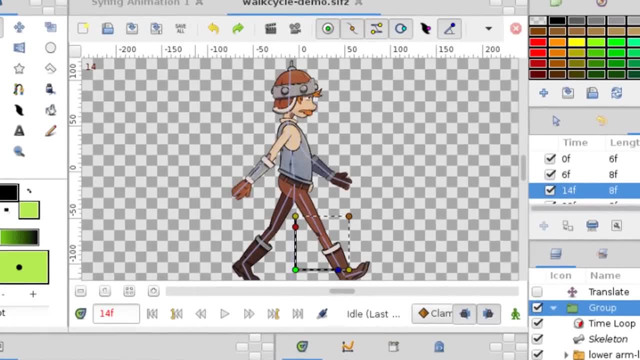 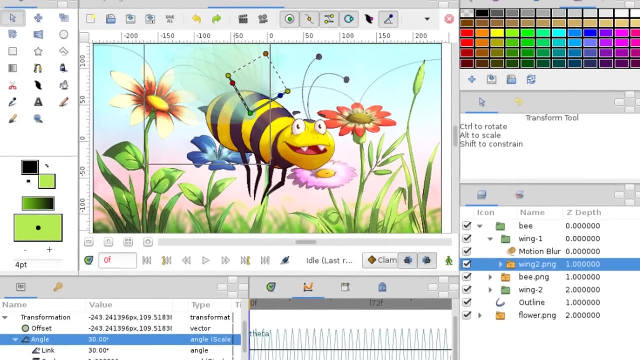 This will lead to time loss, Especially in this period. we don't have the luxury to lose time. We have Sinfig animation software, so that we don't have to lose time. Additionally, it is free, It is supported by all operating system and there are two options. 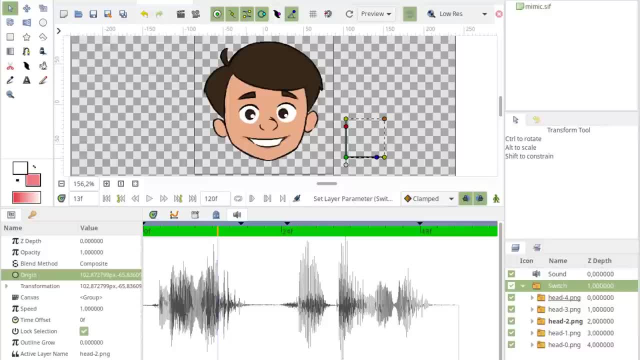 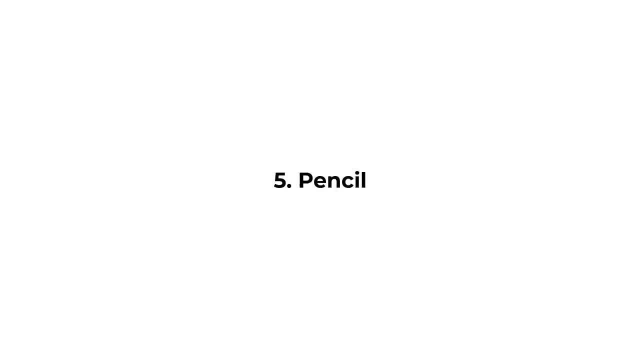 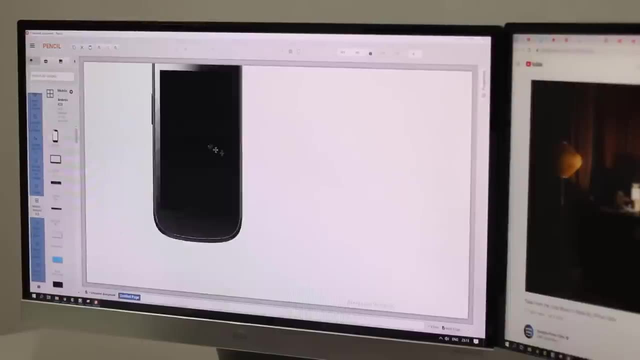 Stable version and Development version. You can go to the official website and download the software. 5. Pencil: The perfect free software to create animated digital comic books. Pencil is a vector drawing program for Windows that enables creating your own digital comics. The software allows you to create your own digital 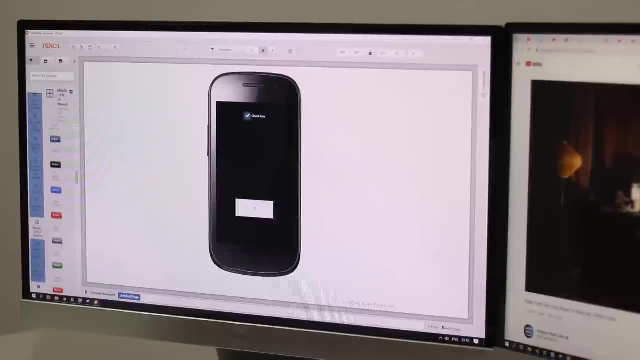 comics, For example. you can create your own comic books using Pencil, and you can also create your own comic books. Pencil is a vector drawing program for Windows that enables creating your own digital comic books. It is based on pen drawing and traditional hand-drawn animation techniques. 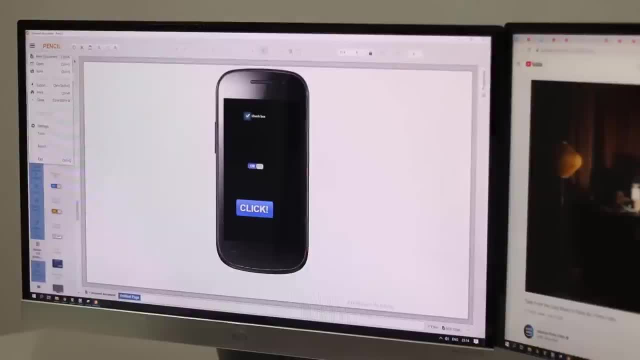 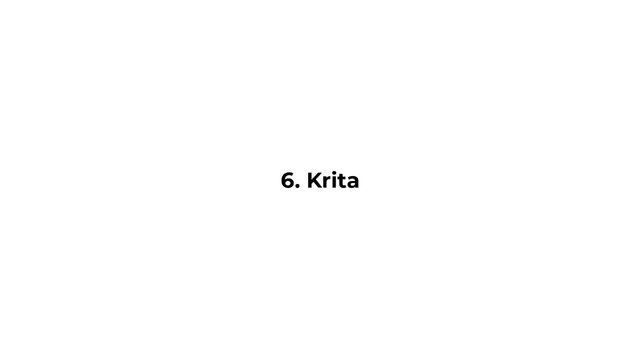 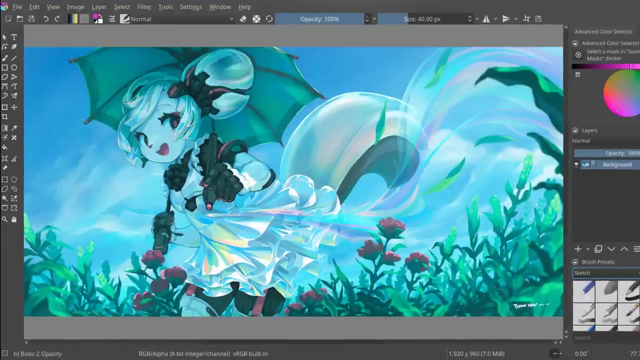 and the software is free. If you are new in animation, you must try Pencil. It can be a good choice for basic work. 6. Krita More than just an animation software. if you have drawing skills, Krita offers practical. 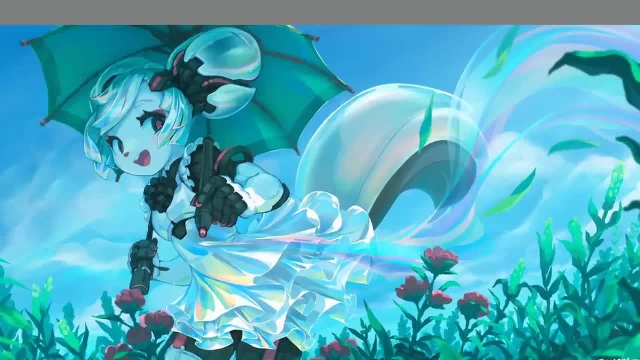 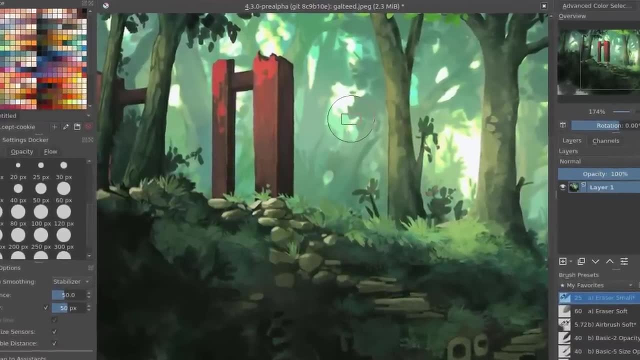 tools and you can make amazing drawings. Of course, if you want your drawings to move, you can turn them into animation. Krita is free software. If you want to support the developers, they have a donation area on their website. You can use this software easily. 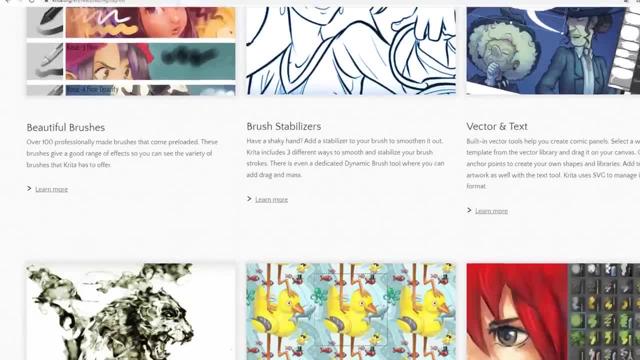 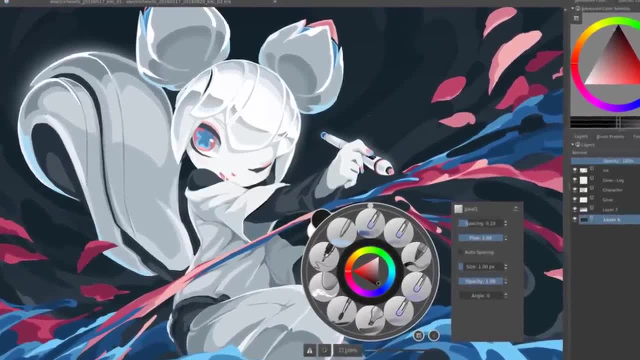 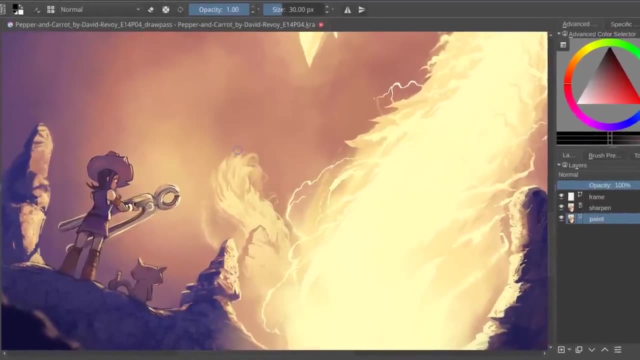 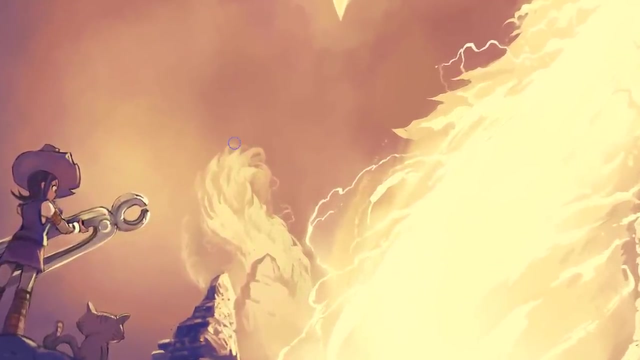 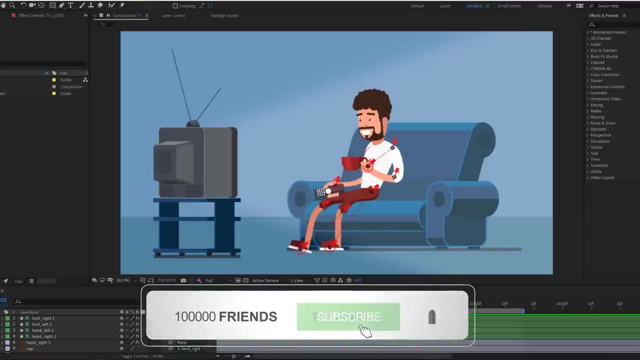 at school or in the workplace. It is an amazing feeling to make wonderful drawings and make them move. You can create your own cartoon and make people watch it. It is simple and practical. 7. After Effects. Everyone knows this software. Someone can say: why After Effects? Because we can do. 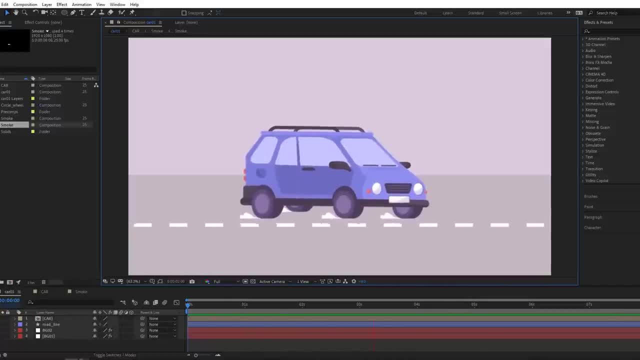 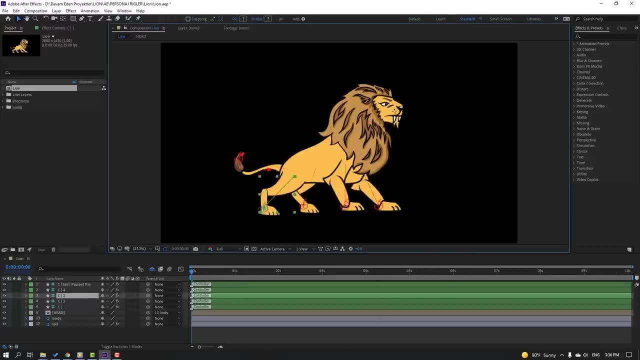 everything with this software, Not just 2D animation. we can do 3D animations, visual effects and motion graphics. There are many character rig making, plugins for After Effects- We can say Dweck and Rubber Horse, as well known. After making the 2D animation, we are 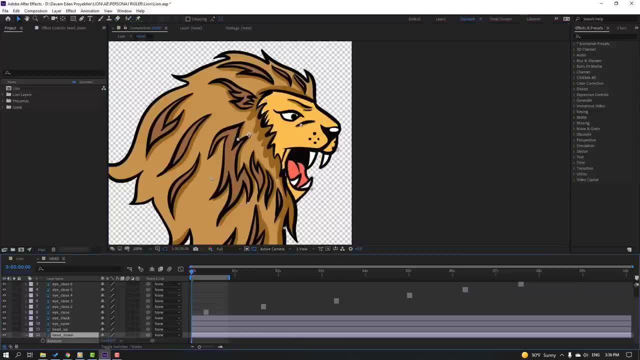 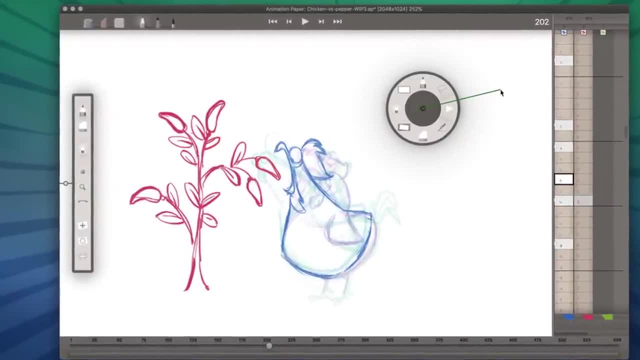 compositing it, and here comes a perfect cartoon 8. Plastic Animation Paper. This is an ideal choice for fast and high-quality work. When we look at their official website, we can see that 325,061 people have clicked on it. This is a great way to make your own. animation 8. Plastic Animation Paper. This is an ideal choice for fast and high-quality work. When we look at their official website, we can see that 325,061 people have clicked on it. This is a great way to make your own. animation. We can say Dweck and Rubber Horse. This is a great way to make your own animation. When we look at their official website, we can see that 325,061 people have clicked on it. This is a great way to make your own animation. 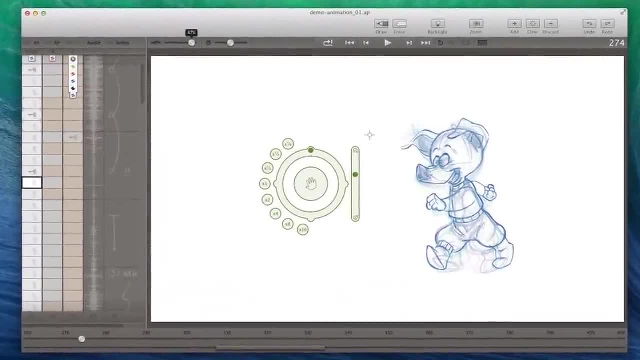 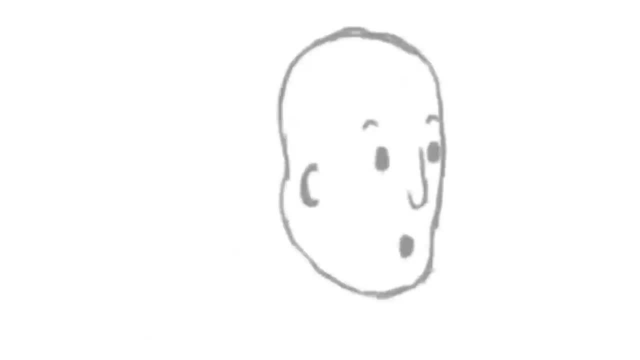 8. Plastic Animation Paper. This is huge and it is perfect for those who make fast and high-quality animation. You can read the blog articles on their website to see how far they have reached. There is always innovation and comfort. They have explained the software on the homepage with 5 properties. 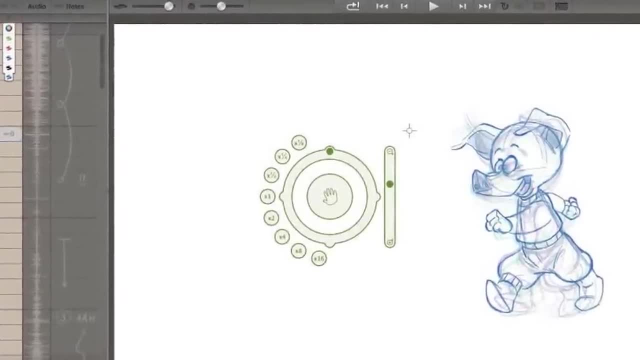 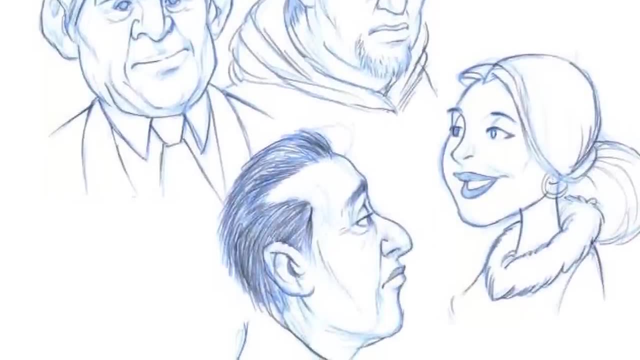 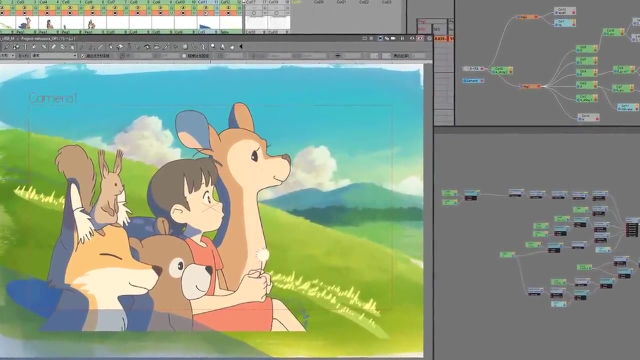 – power, speed, efficiency, easy and simple. I think you should download it now. I am sure it is something worth using. 9. OpenToonz: We can say this is an amazing software to the animation producers, OpenToonz based. 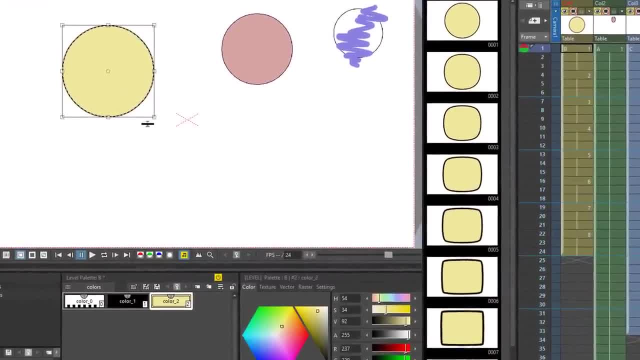 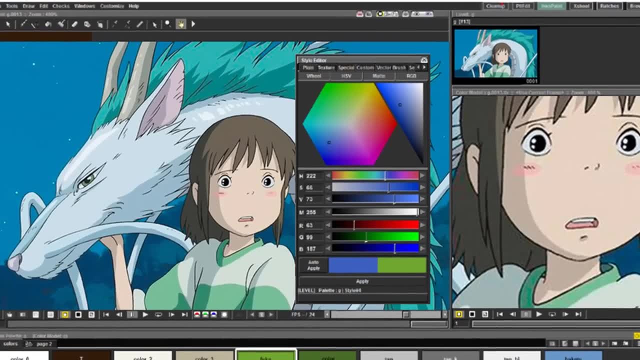 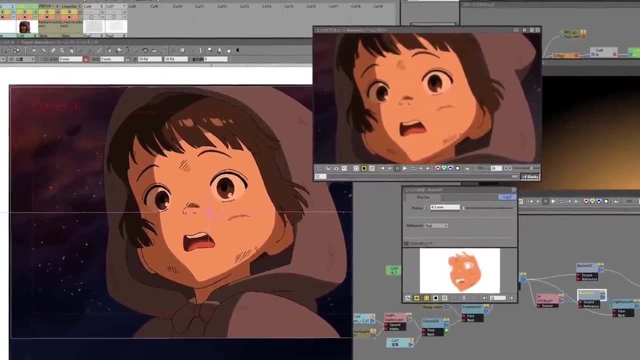 on Toonz. software developed by Digital Video SBA in Italy was privatized by Studio Ghibli, and the software has been used in creating animation work for years. You can use this animation software for free, in both commercial and individual projects. Moreover, it is open-coded. 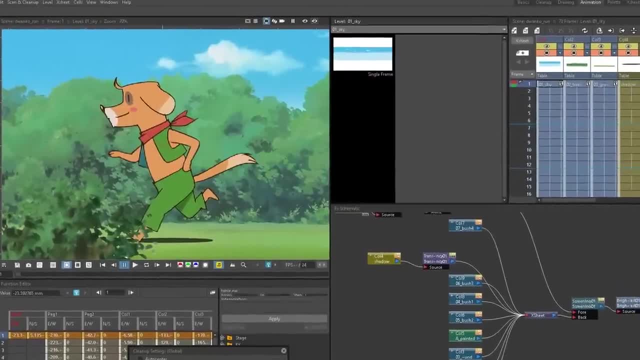 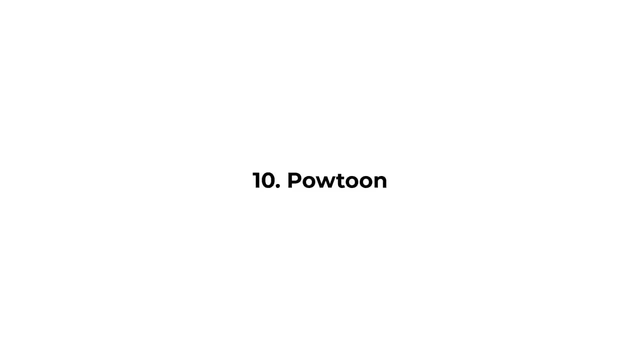 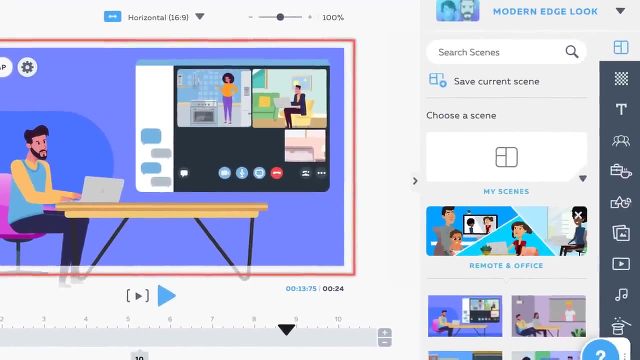 This way, anyone can customize the source code. 9. OpenToonz: If you want to become a professional in animation, you must try OpenToonz. 10. PowToonz: Do you want to make easy and fast animations? Yes, PowToonz is a software that is for you. 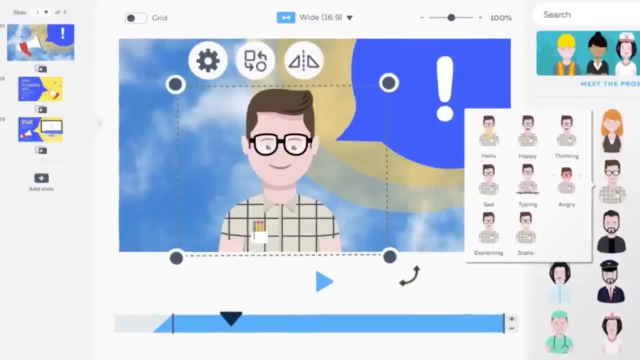 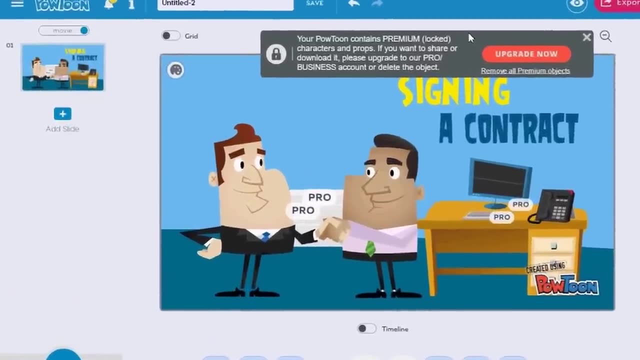 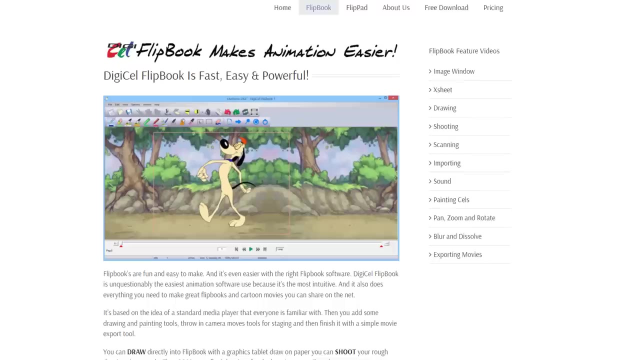 At once. open the software, use its easy interface and make your dream animation. If you are a YouTube broadcaster and you think to produce fast animations, this software is for you. Take it and use it. 11. FlipBook: It is easy to learn and it is very affordable software. The interface is very understandable. 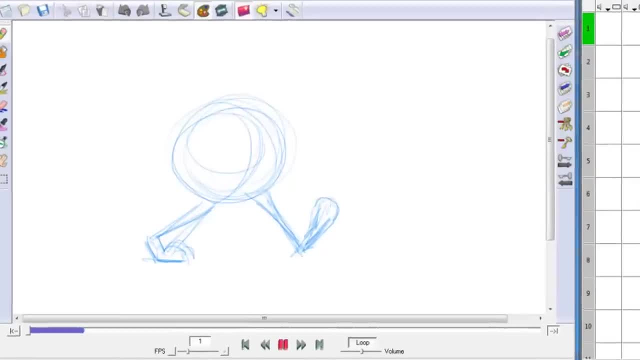 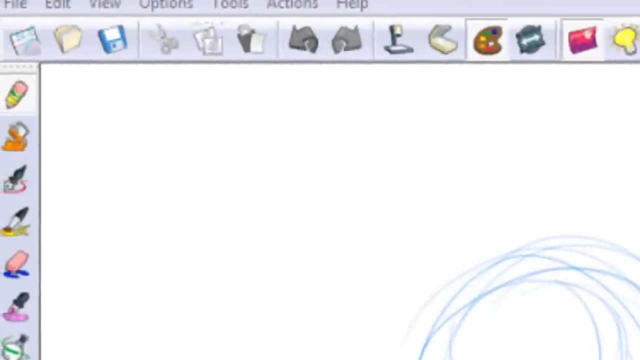 for making animations. You can give a flip to diagrams with drawing them in the software. It is possible to make very beautiful animations with very easy ways. Make sure that you don't need to vary long instructions for use to use the software. Software is very easy. you. 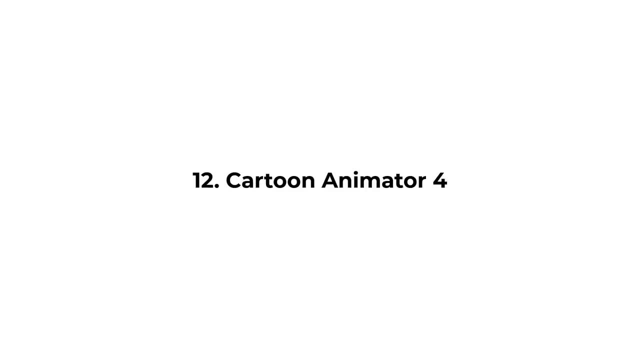 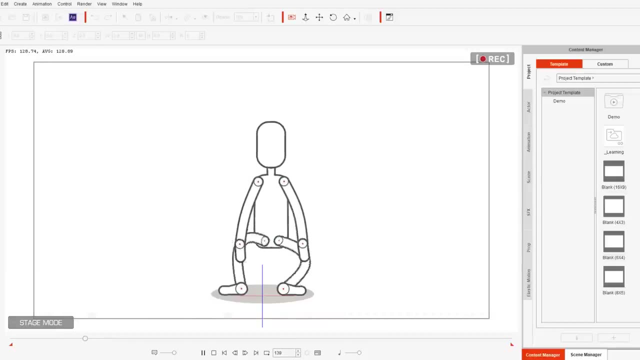 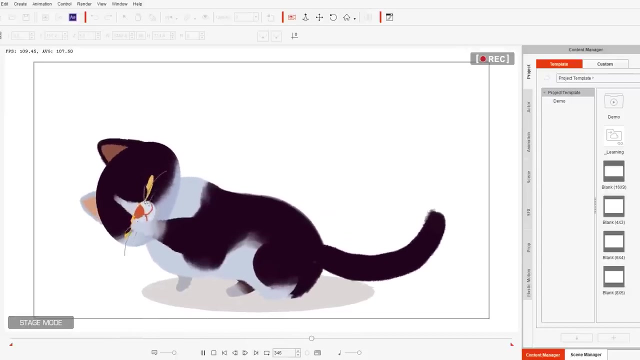 can learn it instantly. Number 12,: Cartoon Animator 4. Cartoon Animator 4, formerly known as Crazy Talk Animator, is a 2D animation software designed for both ability of entry and productivity. You can turn images to animated characters. control characters with your expressions. 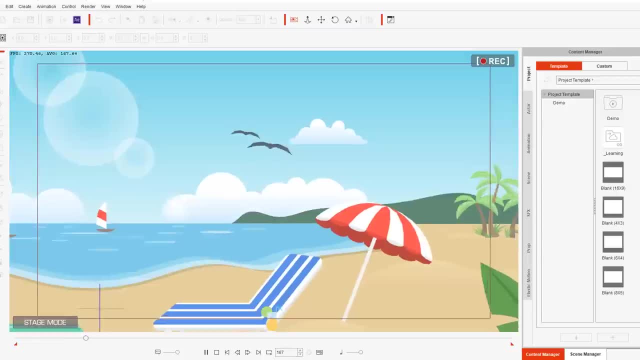 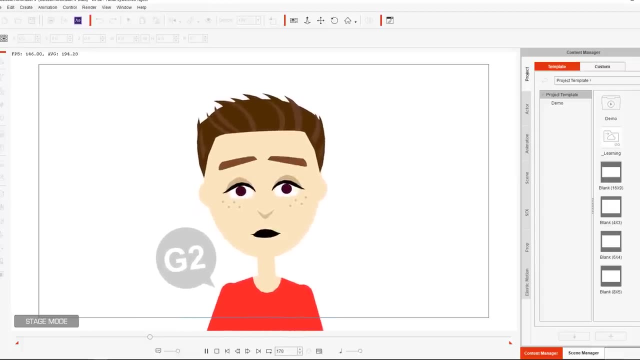 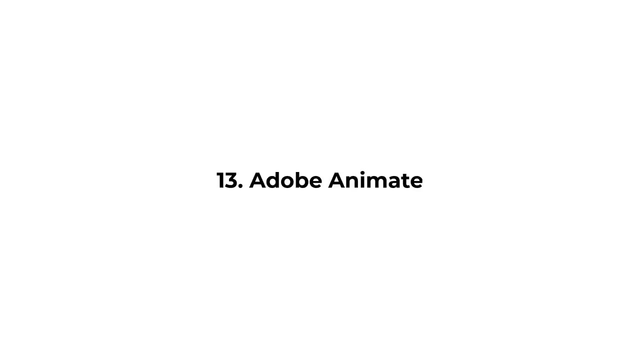 generate lip-sync animations from audio, accomplish 3D parallax scenes, produce 2D visual effects, access content resources and wield a comprehensive Photoshop pipeline to rapidly customize characters and create content. Number 13, Adobe Animate: Animate just about anything. 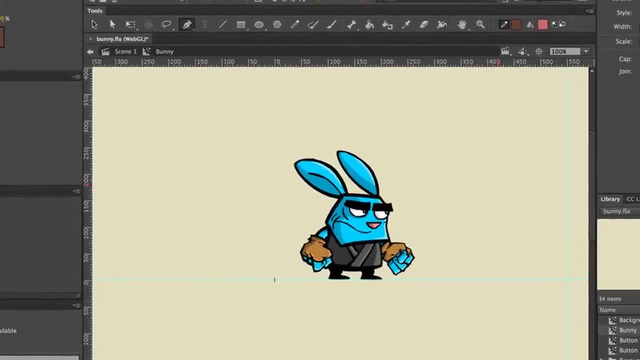 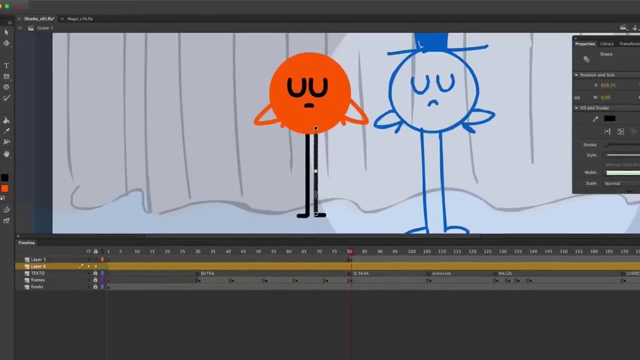 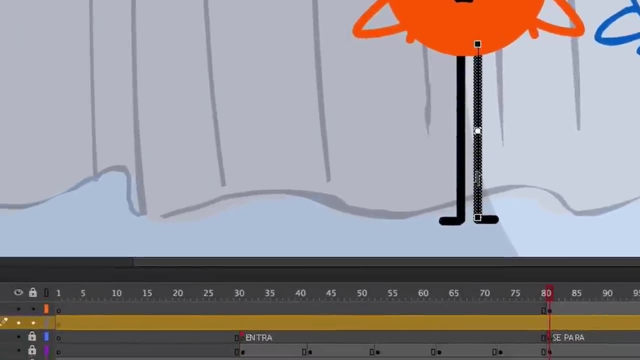 Design interactive animations for games, TV shows and the web. Bring cartoons and banner ads to life. Create animated doodles and avatars, and add action to e-lining content and infographics. With Adobe Animate, you can quickly publish to multiple platforms in just about any format and reach viewers on any. 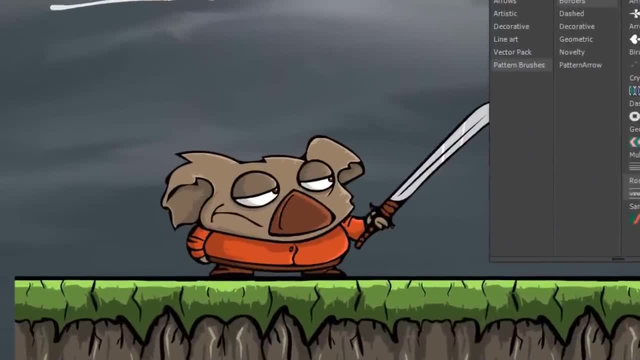 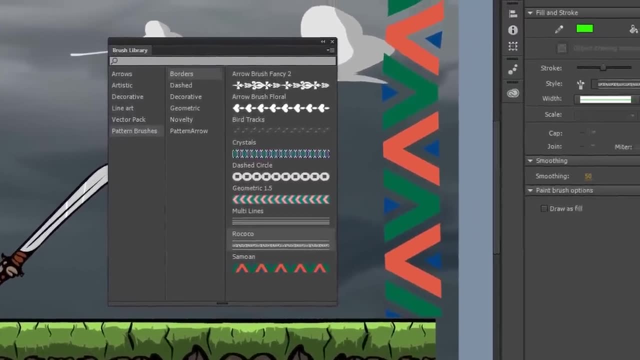 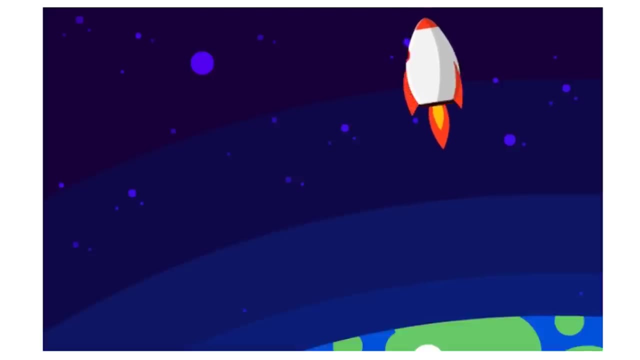 screen. Create interactive web and mobile content for games and ads using powerful illustrations and animation tools. Build game environments, design start screens and integrate audio. Share your animations as augmented reality experiences. With Animate, you can do all your asset design and coding right inside the app. 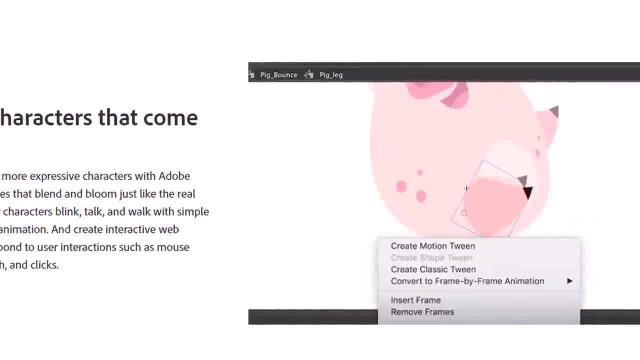 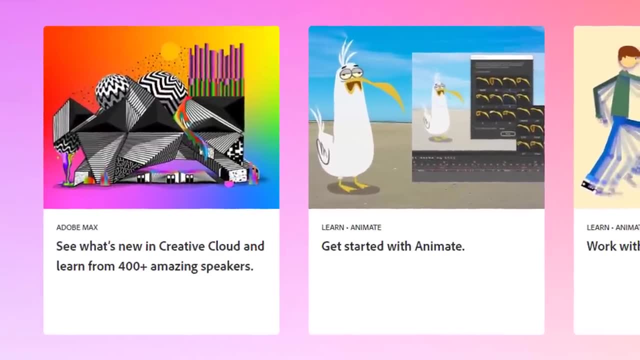 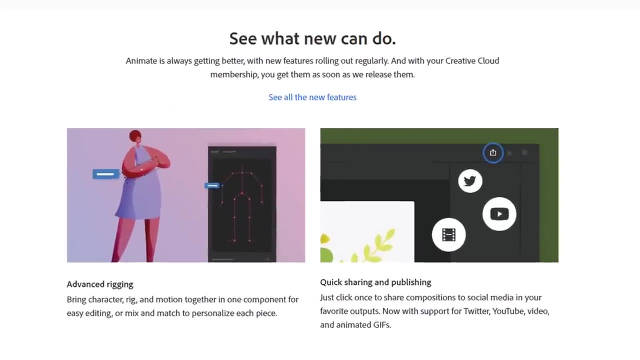 Sketch and draw more Expressive characters with Adobe Fresco live brushes that blend and bloom just like the real thing. Make your characters blink, talk and walk with simple frame-by-frame animation And create interactive web banners that respond to user interactions such as mouse movement. 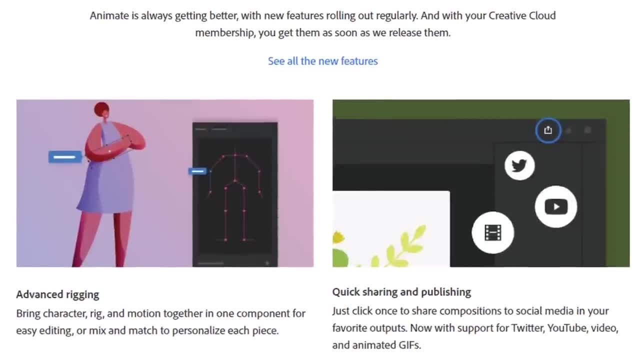 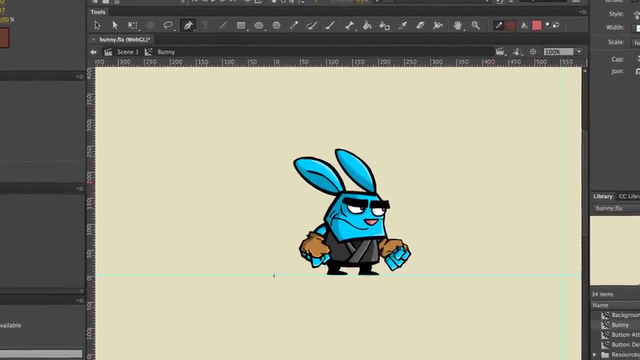 touch and click. Reach your audience on desktop, mobile and TV by exporting your animations to multiple platforms, including HTML5, Canvas, Wordpress and Google Play. You can also create interactive web and mobile animations for games and ads using multiple platforms. 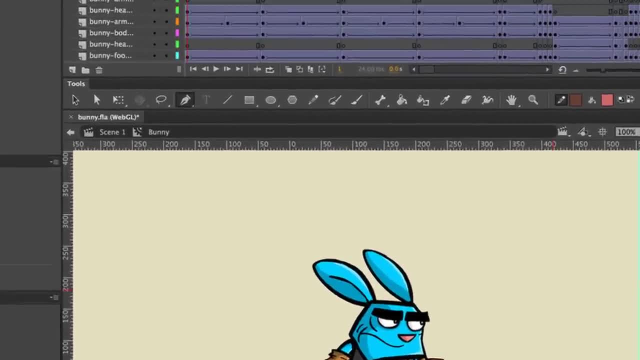 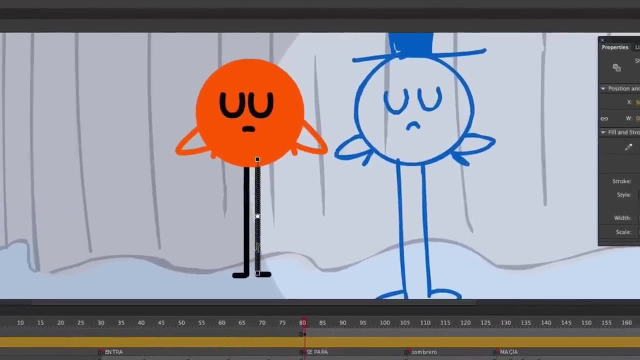 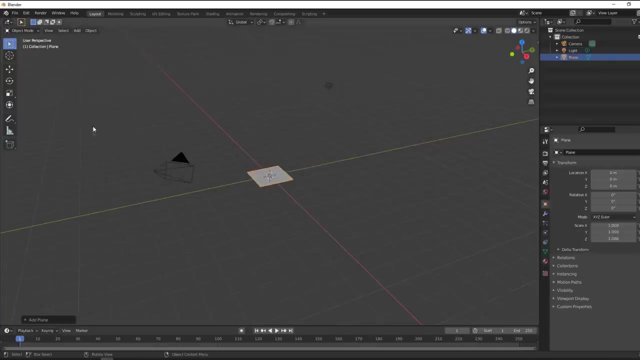 There's Netz A In Sky, Canvas, WebGL, Flash and Adobe AR And custom platforms like SVG. You can include code right inside your projects and even add actions without having to code discipline Blender. Blender is the free and open-source 3D and 2D creation suite. 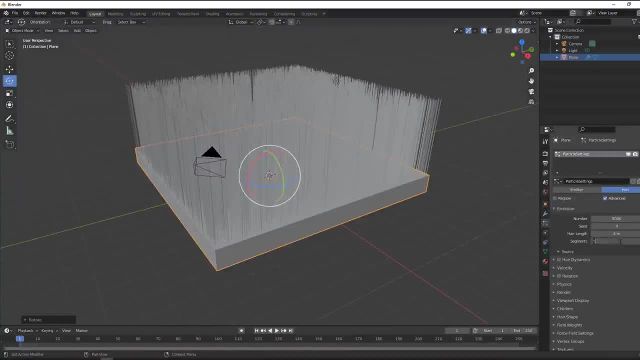 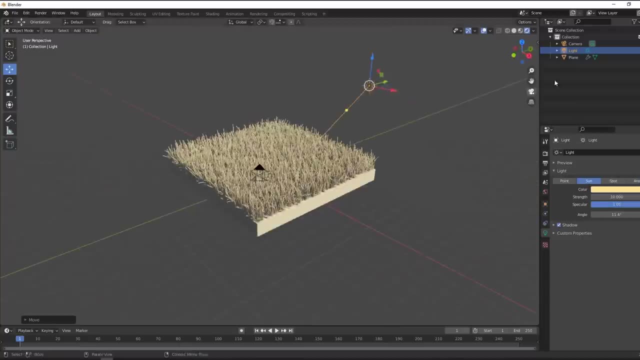 It supports the entirety of the 3D pipeline — modeling, reging, animation, simulation, rendering, compositing, etc. and more. For more help, visit http//wwwblendercom. and motion tracking, even video editing and game creation. Advanced users employ Blender's API for 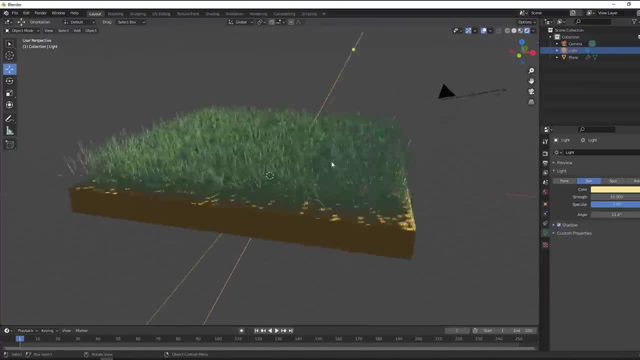 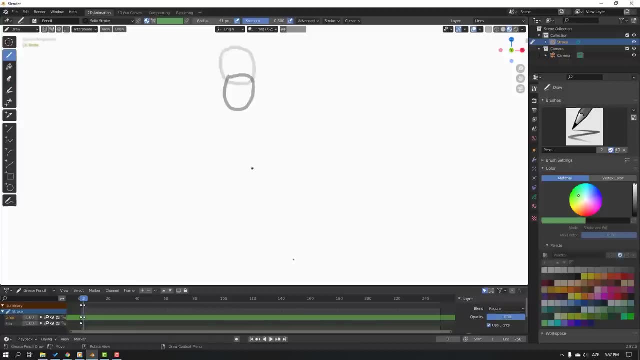 Python scripting to customize the application and write specialized tools. Often, these are included in Blender's future releases. Blender is well suited to individuals and small studios, who benefit from its unified pipeline and responsive development process. Examples from many Blender-based projects are available in the showcase.